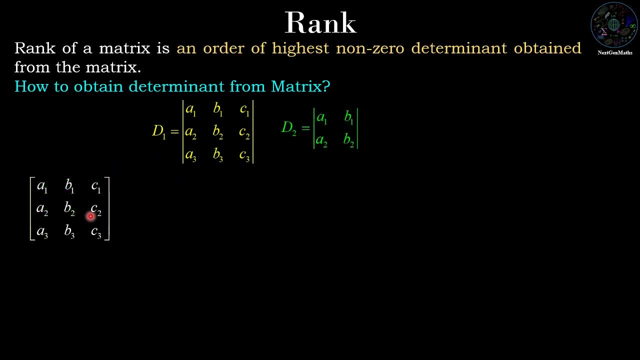 So the second, anytime of order 2 will select first two rows. we select first two rows and first three columns will give the another determinant of order order 2: a1, c1, a2, c2. then first two row and second and third column will give. 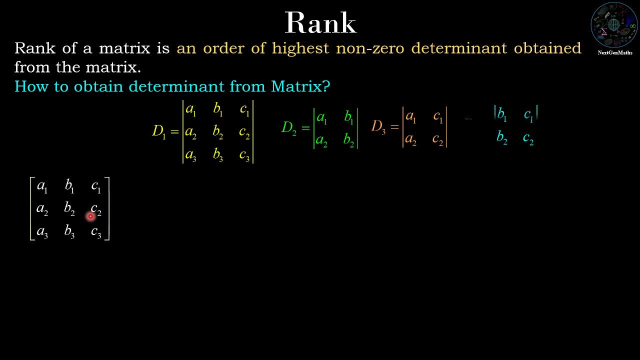 the another determinant, b1, c1, b2, c2, of order 2.. So from first two row we are able to generate three determinant of order 2.. Now we select another two row, first and third row, with the intersection first and second column. then we have a1, b1, a3, b3.. Next, first and third row and first and third column. 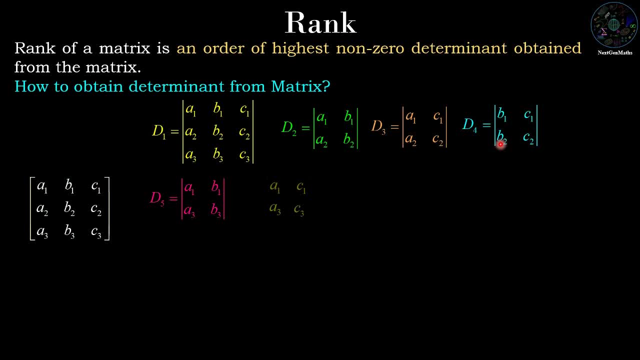 will give a1, c1, a3, c3.. First and third row and second and third column: b1, c1, b3, c3. Now we select another two row, second and third row. then it will give the next determinant: a2, b2, a3, b3. then select first and third column. intersection with: 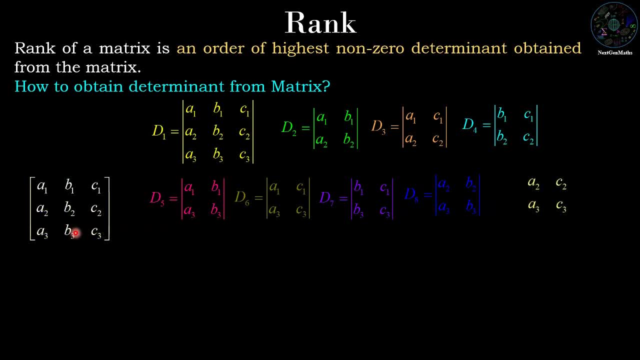 the second and third row, so a2, c2, a3, c3, then second and third row. second and third column will give the determinant of order two: b, 2, c2, b, 3, c3. Now we cannot find any other determinant of order two. therefore we are going to. 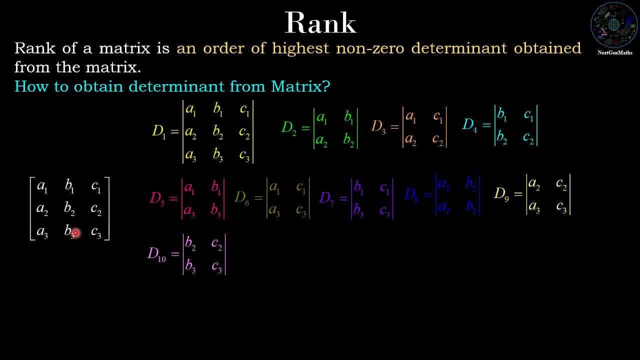 find the determinant of order one and we have nine entries, so nine determinant of order one, C1, A2, B2, C2, A3, B3, C3 and total 19. determinant we can obtain from the cross 3 matrix. 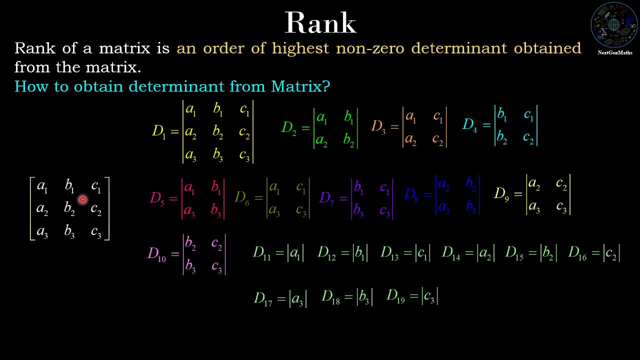 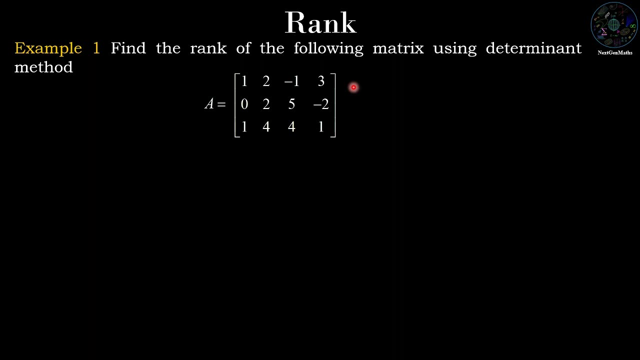 and the order of highest non-zero determinant from this determinants will give the rank of a matrix. Example: find the rank of the following matrix using determinant method: The given matrix is of order 3 cross 4.. So largest determinant obtained from 3 cross 4 matrix is the 3.. 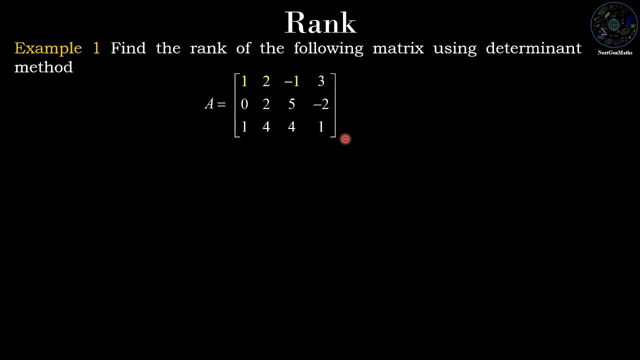 So for that we select first 3 column, We will get the first determinant of order 3.. Say D1 and we are going to evaluate the determinant, So 1 multiply with its minor, Then 2 multiply with its minor and minus 1 multiply with its minor. 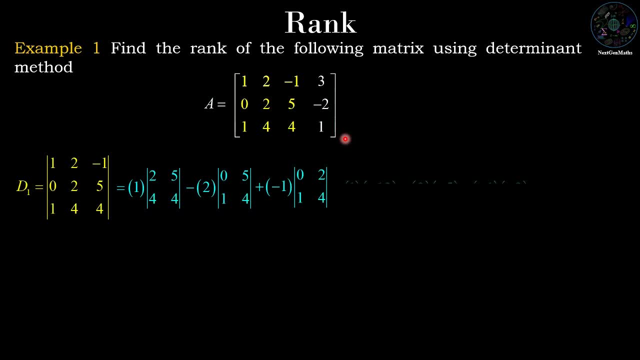 Then we have 1 multiply with 8 minus 20, which is minus 12.. 2 multiply with 0 minus 5, minus 5.. Minus 1 multiply with 0 minus. Then we have 1 multiply with 0 minus 2, and its value is 0.. 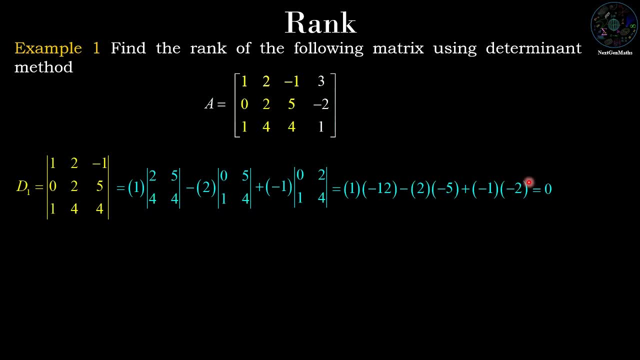 So D1 has value 0, but we want non-zero determinant, So we are going to find the another determinant of order 3, if it is possible. So if we select first, second and third column, then we are able to generate another determinant of order 3.. 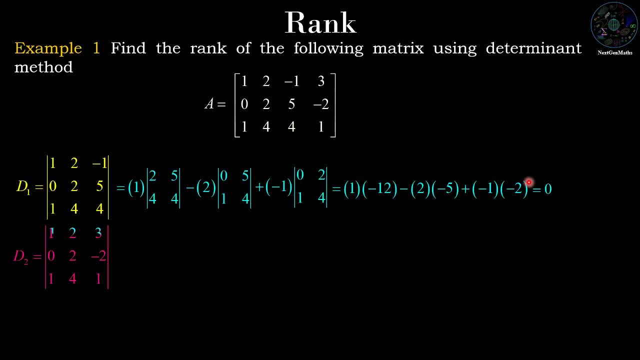 Now we evaluate determinant D2.. So multiply 1, 2, 3 with its minor, Then we have 1 multiply with 2 plus 8, 10,. 2 multiply with 0 plus 2, 2 and 3 multiply with 0 minus 2, which is also 0.. 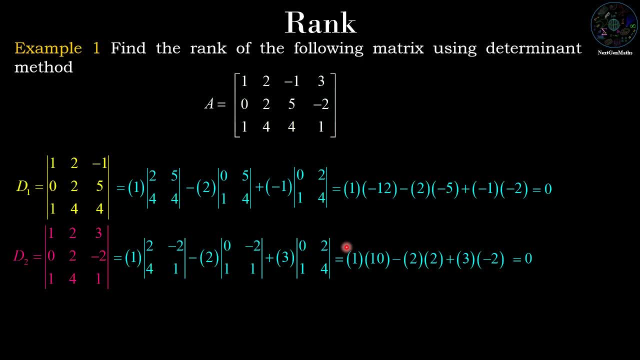 So we are going to find the another determinant of order 3 by selecting first, third and fourth column And we are going to evaluate 1 minus 1, 3 with its minor. Then the corresponding value is also 0..